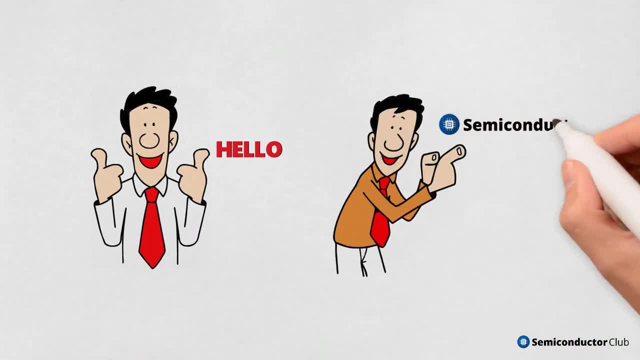 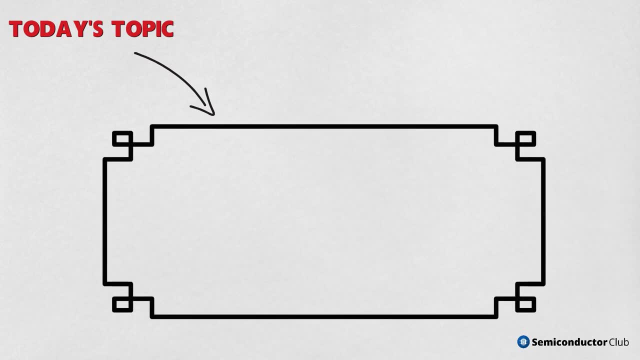 Hello and welcome to Semiconductor Club, where all we talk about Semiconductor Engineering. Please show a thumbs up and subscribe to our channel. In today's topic, we will learn about what is ASIC, FPGA and SOC and the examples regarding this. Let's start with an application-specific integrated circuit- ASIC, As the name suggests. 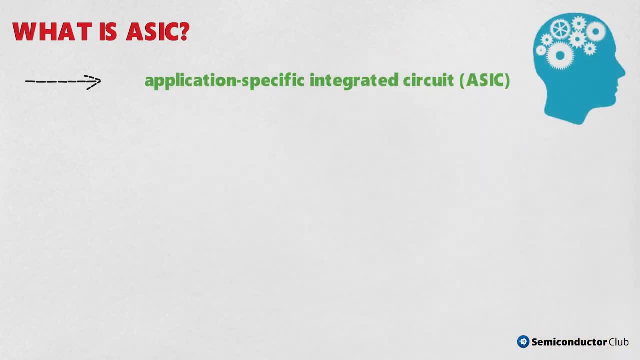 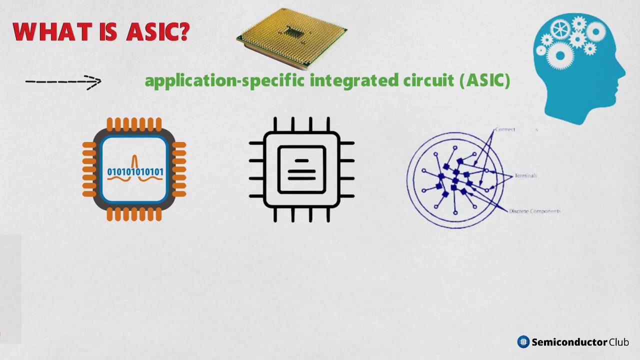 this is a device that is created with a specific purpose in mindAny chip that is custom made is an ASIC, irrespective of whether it is analog, digital or a mix of both. ASICs are typically designed and used by a single company in a specific system. They are incredibly expensive. 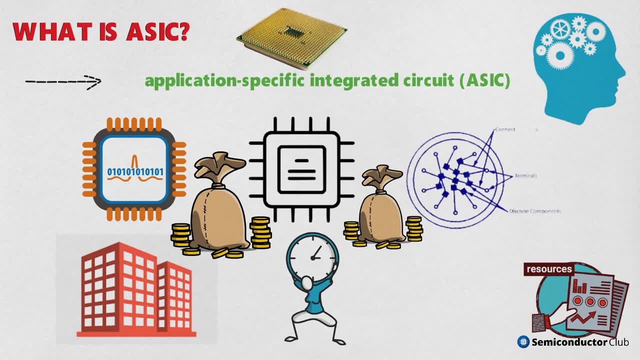 time-consuming and resource-intensive to develop, but they do offer extremely high performance coupled with low power consumption. Example regarding this is a 24x2410G Ethernet switch that is custom designed for a specific system to meet performance, power demand, sec. 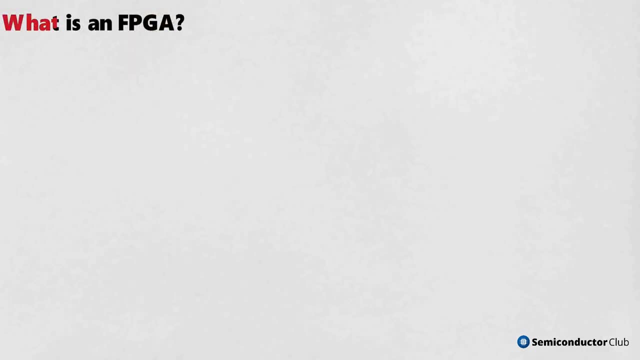 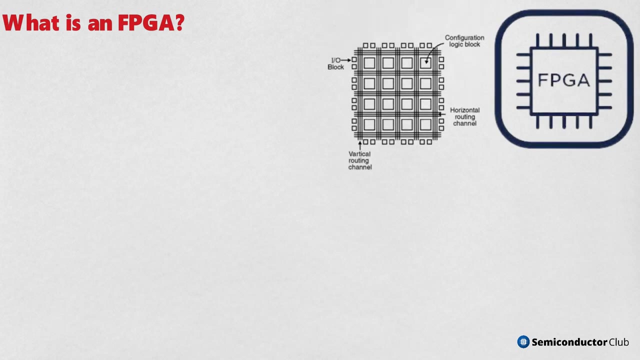 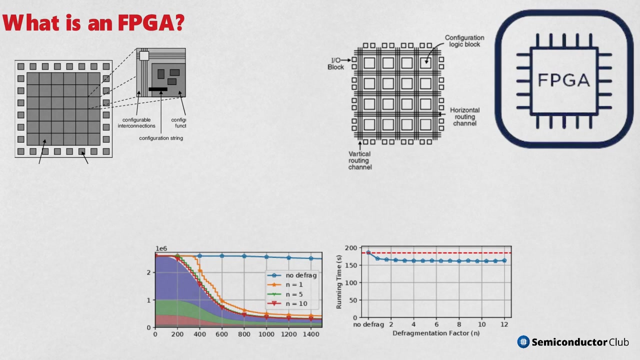 FPGA. The architecture of early FPGA devices was relatively simple: just an array of programmable blocks linked by programmable interconnect. The great thing about an FPGA is that we can configure its programmable fabric to implement any combination of digital functions we desire. Also, we can implement 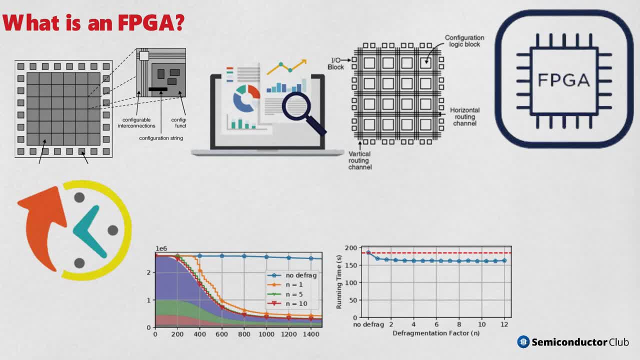 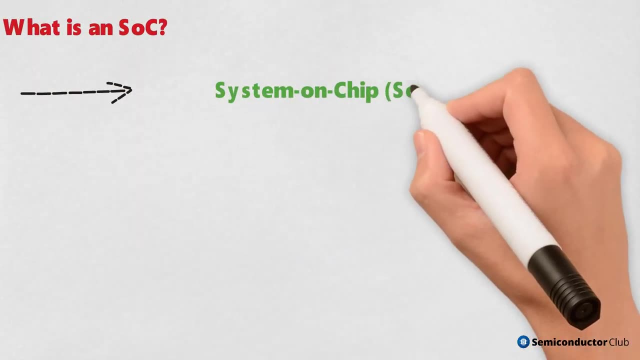 algorithms in a massively parallel fashion, which means we can perform a humongous amount of data processing very quickly and efficiently. Example of an FPGA is Xilinx, Spartan and Vertex series. How to Align a Late Ch решet. So let's be frank. this year the SOC. a system-on-chip, is a silicon chip that contains one or more processor. 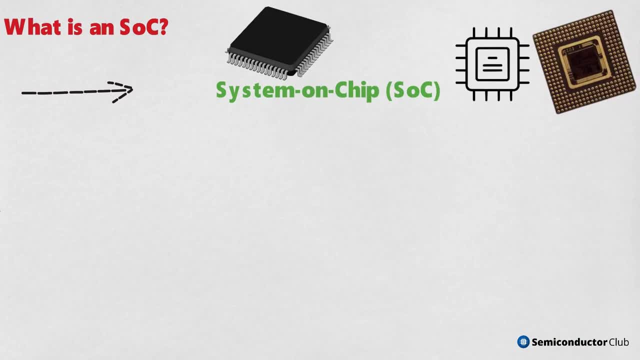 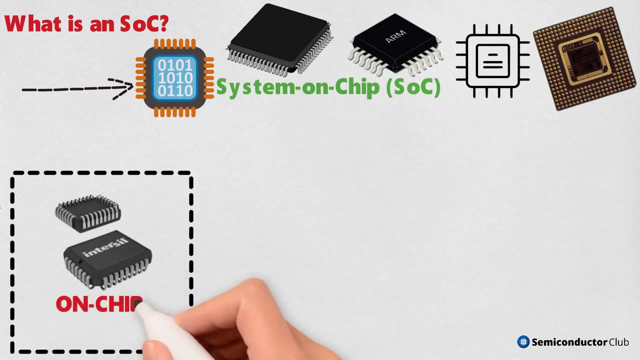 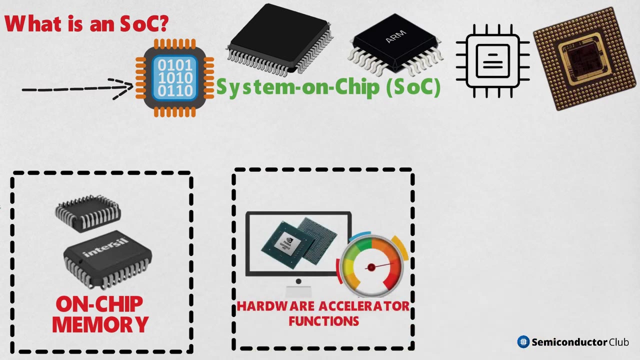 cores, microprocessors and or microcontrollers and or digital signal processors, along with on-chip memory hardware, accelerator functions and potentially all sorts of other stuff. One way to look at this is that if an ASIC contains one or more processor cores then it's an SOC. Similarly, Hroz палbandı ​​ Australia's Cortesī tomorrow will theme this. A must-have have, in the corporate community. It is frequently chucked to the Hordo website. Be sure to visit USAS to get any of these meiner thiчикórde queries, or coconicketyan�il 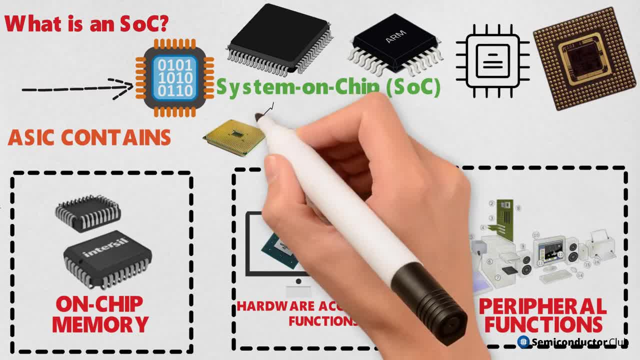 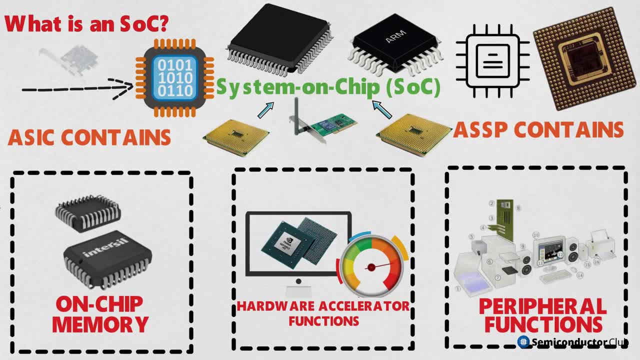 if you've made any minor work on the course. This two days may not exceed one to ten. Similarly, if an ASSP contains one or more processor cores, then it's an SOC. We can think of Ethernet Controller, PCIe Controller, SATA USB when we hear the word. 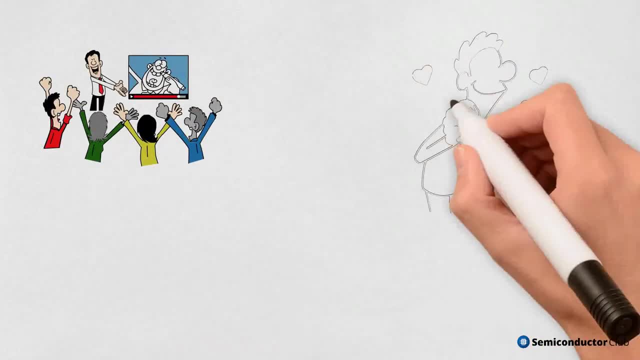 SOC. And that was it for today. guys press that bell icon so you never miss any future videos. see you in the next one. Thanks for watching.